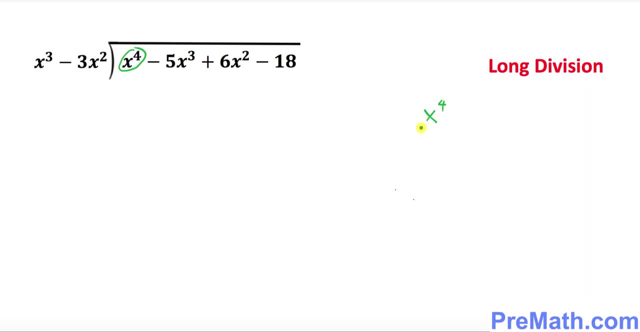 write down x power 4 right up here, divided by the leading term outside, which is divisor, which is x power 3.. So that's going to give us x. So I want you to put down that x, whatever this thing, right up here, and then multiply this x with the both term outside. 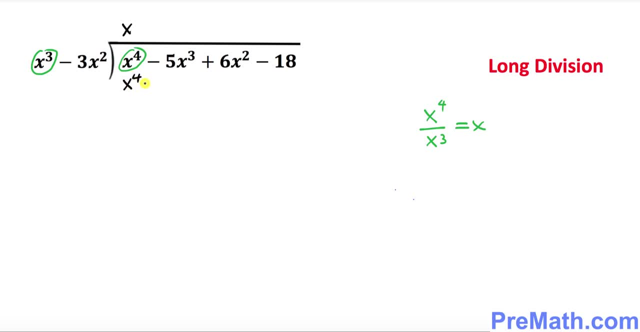 That's going to give us x power 4 minus 3 x power 3.. The next thing, what I want you to do, is I want you to switch the sign So this positive become negative, and I want you to put down x power 3.. So that's going to give us x power 4 minus 3 x power 3.. 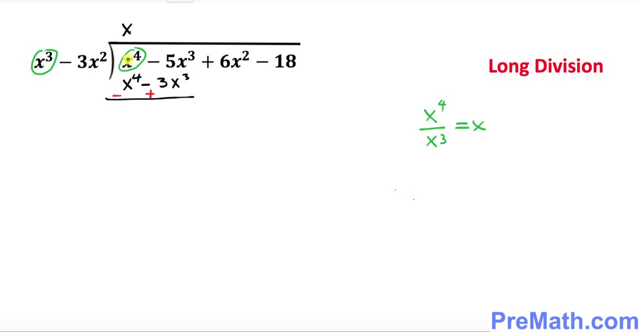 negative become positive. we change the sign. so this is gone. so we got this thing. which is what? negative 2x power 3- I want you to bring these two terms down- which is plus 6x square minus 18. now, once again, I want you to look at this. 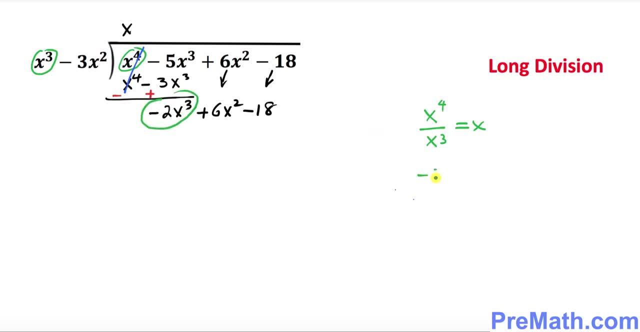 the leading term, which is negative 2x power 3. divided by the leading term over here outside is x power 3. when you simplify or divide, that's gonna give you negative 2. I want you to put this negative 2 right up here and multiply. 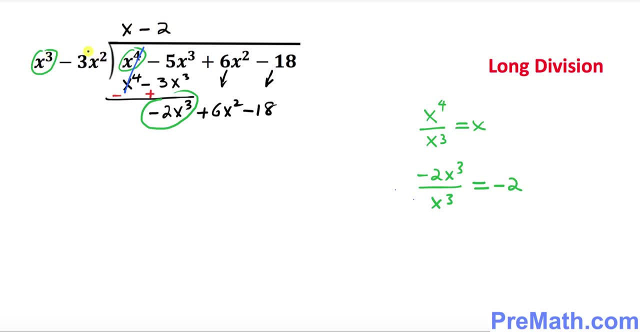 this negative 2 with the both term outside. so that's gonna give you negative 2x power 3 plus 6x square. once again, I want you to change the signs so this negative become positive, positive become negative. the next thing is you cancel this one out. this is gone. so we ended up with just negative 18 as our 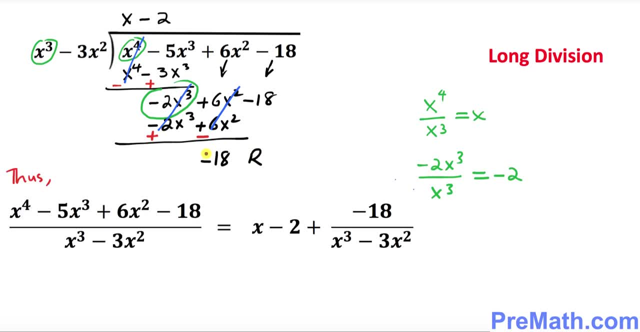 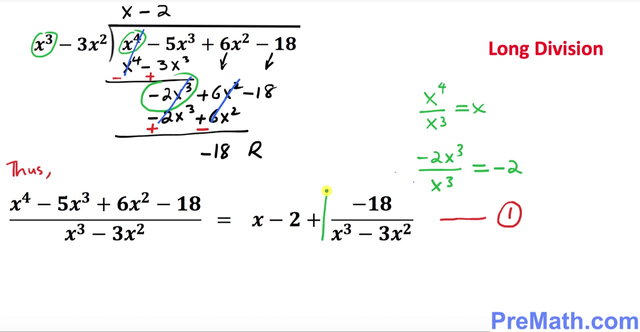 remainder. thus, after the long division, our original equation can be written as this form. all right, so we're gonna call this equation as number one. just keep in your mind now, our next step is going to be performing our partial fraction, only this fraction. this is the rational part. just keep in your mind. 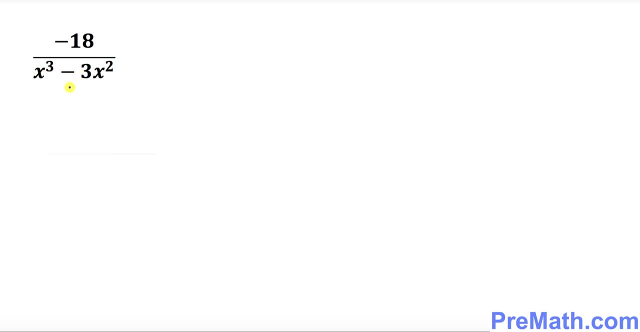 now this fraction could be written as at the denominator. we can write as negative 18 and at the denominator. look at it, what is in common, what could be factored out, and you can see that x square is common. I can factor it out. we got x minus 3. 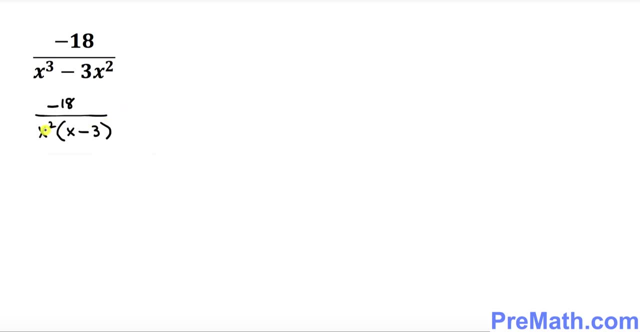 alright. so we got, as a matter of fact, we got x squared and then x minus 3. both are the linear and then x squared. So how we can set it up in a partial fraction, I'm going to put down a over x plus b over x squared. since these x squared are repeated, you just write it in this: 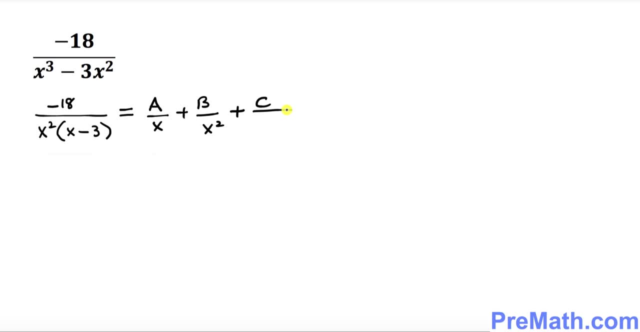 form, and then plus c over x, minus 3.. All right, so once we put it down, this thing, we want to make sure that we get rid of these fractions. So how you can get rid of these fractions. So this is the. 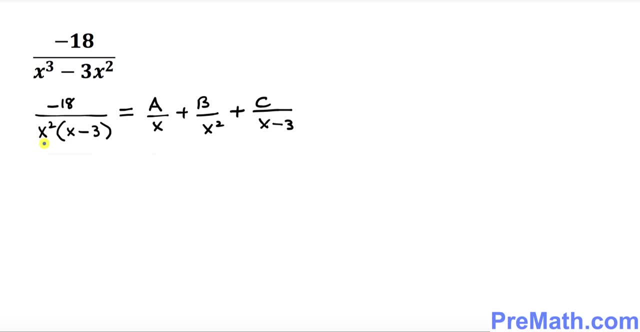 way we're going to do this thing. I want you to multiply whatever is on the bottom across the board: This is x squared- I'm going to put it in this form- and then plus c over x minus 3.. So write down x squared times x minus 3,. I want to write down x squared times x minus 3, x squared. 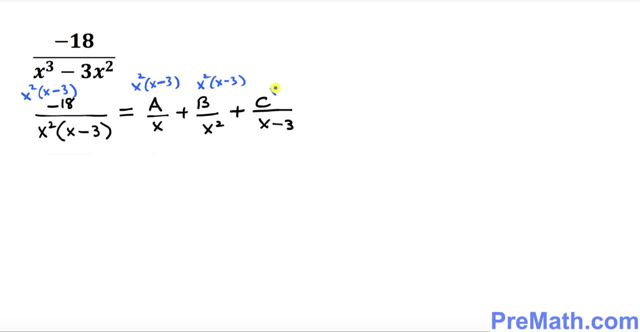 times x minus 3, and x squared times x minus 3 across the board. Now, one thing: you can just see that one this x minus 3, x minus 3, cancel out. this cancels out. So what we ended up with. 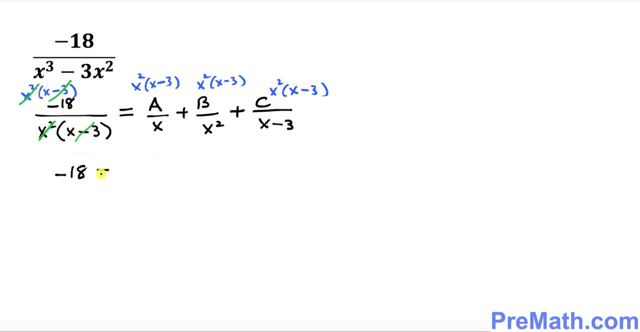 we ended up with negative. We added a positive 18 on the left hand side and on the right hand side. one more thing: You can see that with this one x cancels out. so we simply got what a times x, times x minus 3, and then this x squared cancels. with this x squared, we got plus b. 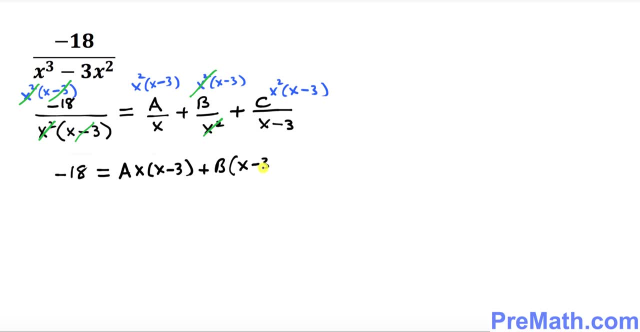 times x minus 3.. and then this thing cancel with this thing. so we got c times x squared. so now we're going to find the value of a, b and c to do that one. here is the simple trick. i want you to just look at the. 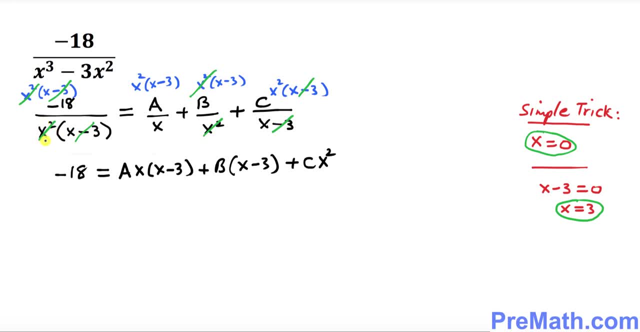 denominator over here on the left hand side. we have a x over here and then we have a x minus 3. i want you to set both equal to 0, so that means we got x equal to 0 and if you set x minus 3 equal. 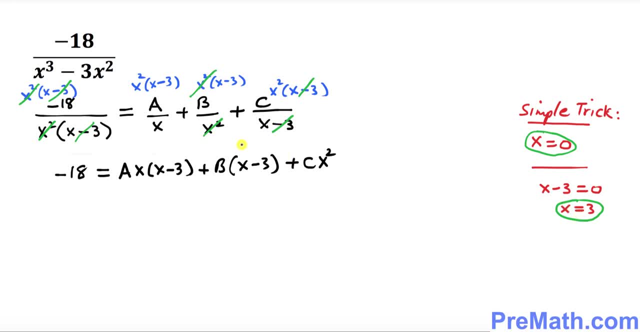 to 0. we got x equal to 3, so we're going to go ahead and and put these one as this one over here. i'm going to put down x equal to 0 first. what is going to happen if i plug it in? x equal to 0? 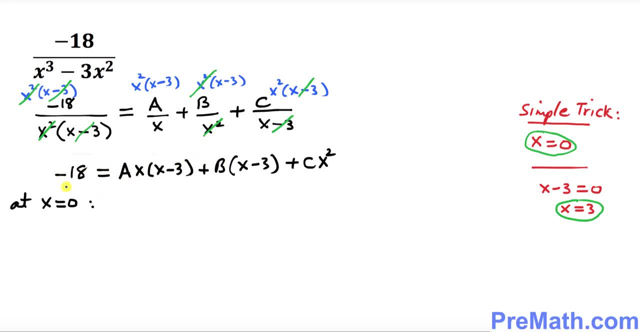 in this, our equation over here. so we got negative 18 on the left hand side, equal to. you can see a times this, 0 times this whole thing. they become a times 0 plus b times 0 minus negative 3 become negative 3 plus c times 0. 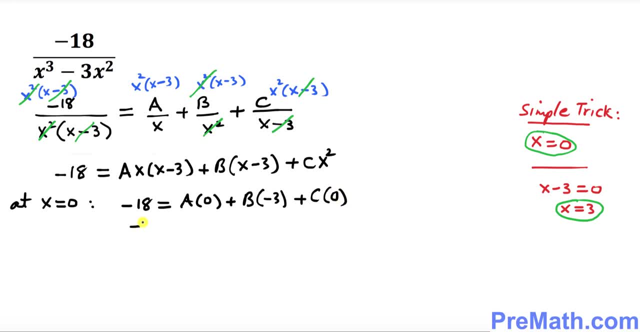 square is 0, so that means we simply got negative 18 equal to negative 3 b, which gives us b equal to 6. so we figured out our b value as 6. now at at x equal to next value is: if you look at on the right hand side, we put x equal to 3. what happens at x equal to 3. so the left hand. 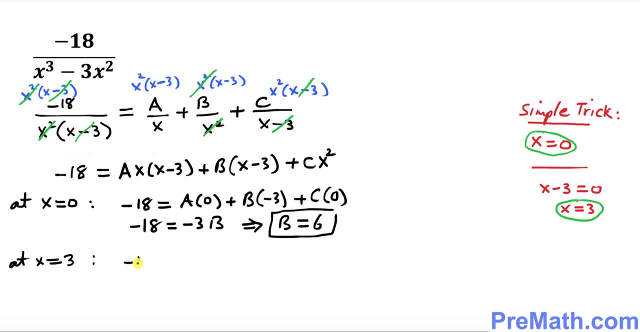 side on, this original equation is going to become negative. 18 equals to 9x plus. we replace this with the 2x plus 8 and so you get negative 18 square, which is going to third plus 3 by dot plus stars. so this is going to become a 10 to the. 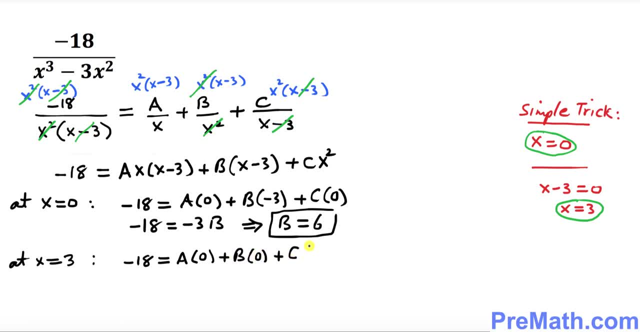 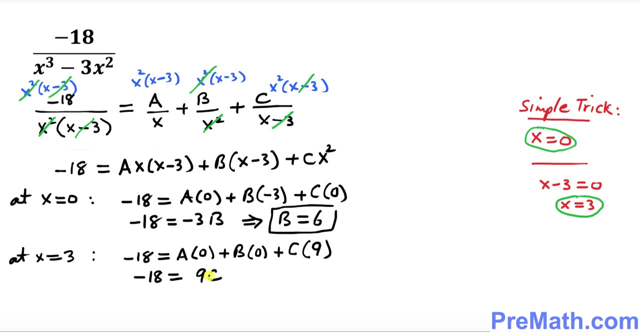 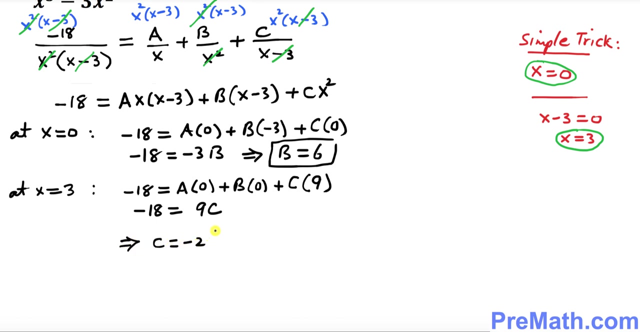 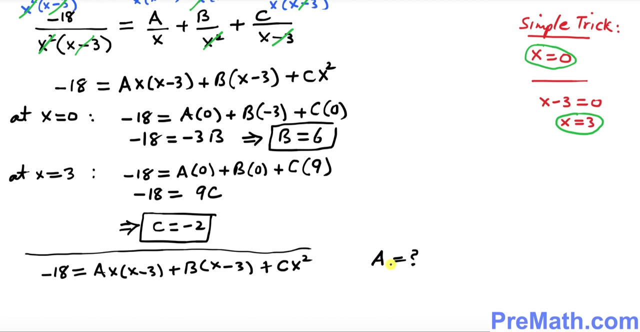 right hand side minus b, square, square, and we end up with b to the left and if you plug it in, x equal. so I just put down 9. so that means we got negative 18 equal to 9 C. so that is going to give us C equal to negative 2. so the next step: we need to find the 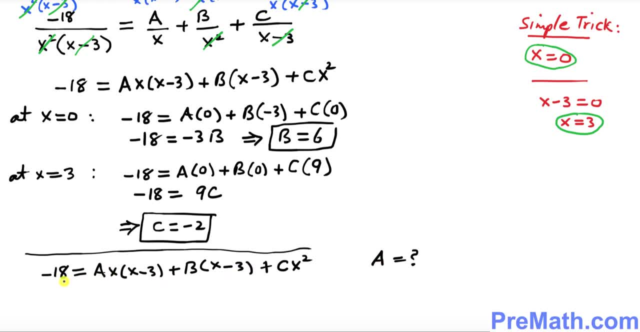 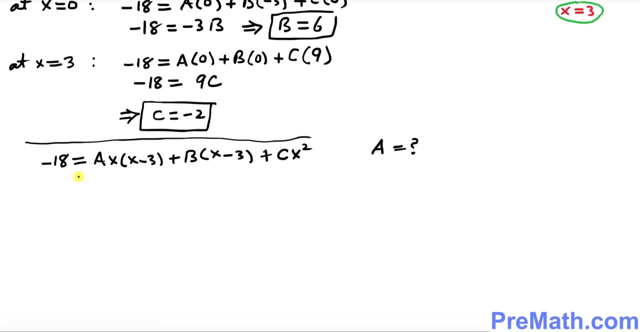 value of a on this equation. so there's no way that we can find this way the easy kind of way. so we're gonna be performing a little bit different way. okay, so you just see how I'm gonna do. I will be using this technique so negative. 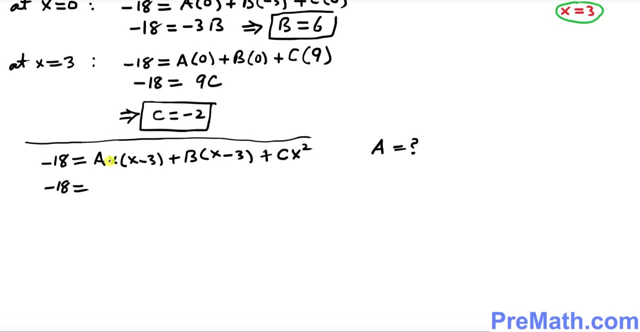 18 equals to here. I want you to just multiply, distribute so this simply become a times x square minus 3x, isn't it? and this is plus B times x minus 3, plus C x square. so let's do this thing over here. I want you to just look at. 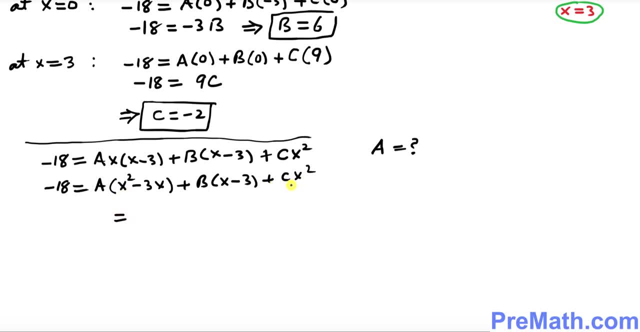 this x square and this x square. see, right now, over here I can write this one, over here I can, so let me just go ahead and distribute it, okay. how about this? okay, so let me just go ahead and distribute it. okay. how about this one? a x square minus 3. a x plus B x minus 3, B plus C x square. and we got. 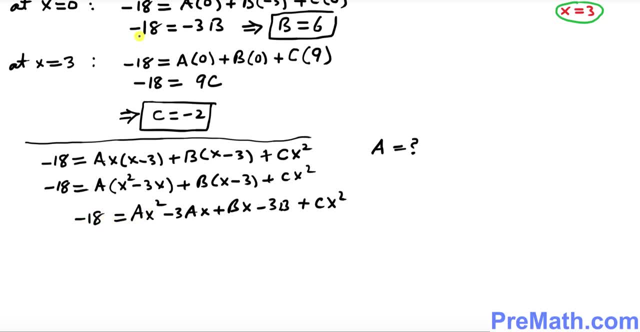 negative 18 still outside. now I want you to just look at this thing: over here, our x square part, this is our x square and this is our x square. can we write this one, as I can write a plus C times x square outside. likewise, over here, I'm gonna write this thing. 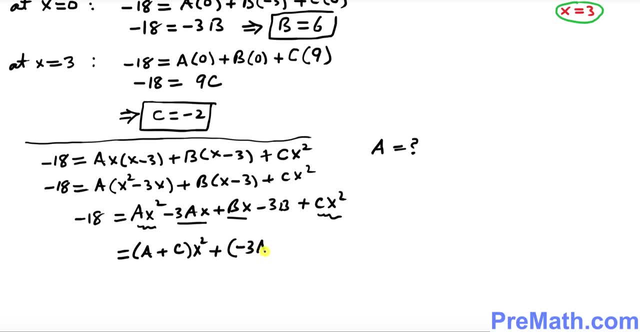 plus negative 3 a plus B times x and plus, and then negative 3 B on this side. okay, so we got this thing, and here we have a plus C times x, square outside. likewise, over here I'm gonna write this thing: plus negative 3 a plus B times x and plus, and then negative 3 B on this side. okay, so we got this thing and here we have a. 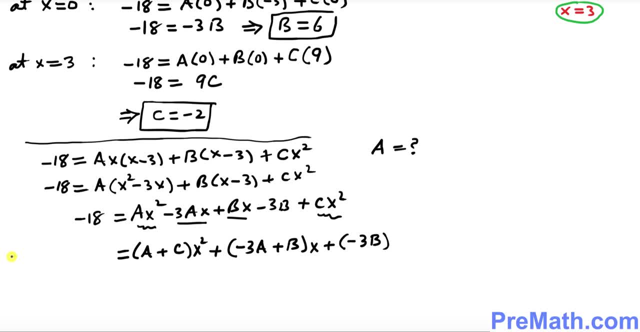 plus C times x square outside. likewise, over here, I'm gonna write this thing plus negative 3 a, plus B times x and plus, and then negative 3 B on this side. okay, so we got this thing and here we have a x square and x is missing. I can write 0x square plus 0x minus 18, and now we're going to be. 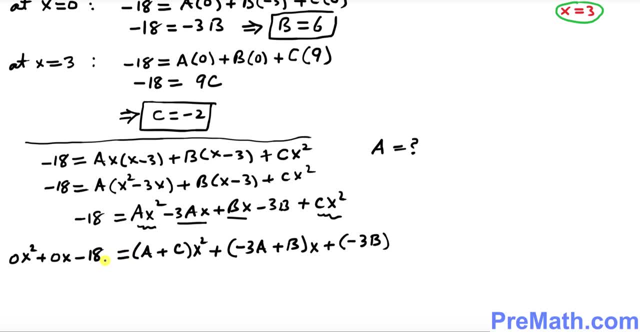 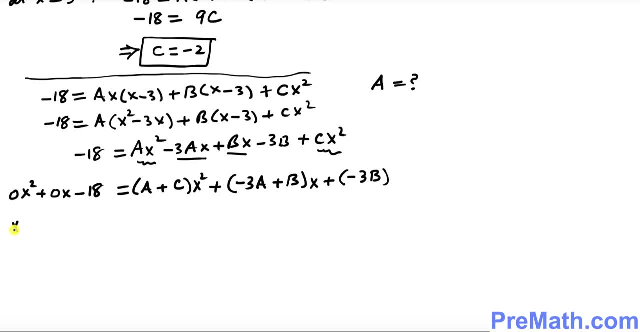 equating the coefficient of x square x and the constants, if we equate the x square part. so what we're going to do is so x square for x square. what happens we got. on this side, the coefficient for x square is 0, equal to the. on the right hand side, the coefficient of x squared is a plus c. so we got. 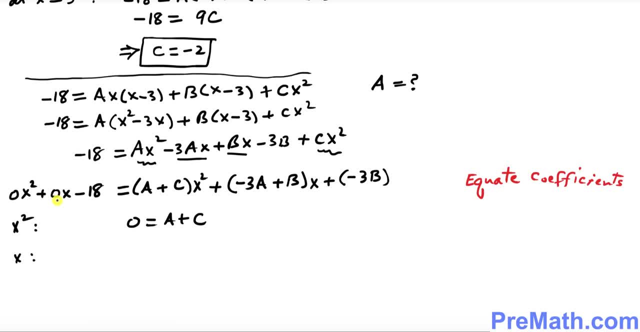 one equation: how about for x? it's going to become 0, equal to negative 3a plus b, and we're going to be equating the coefficient of x square x and the constants. if we equate the, finally, for the constant term, constant term, what you got? negative 18, equal to. 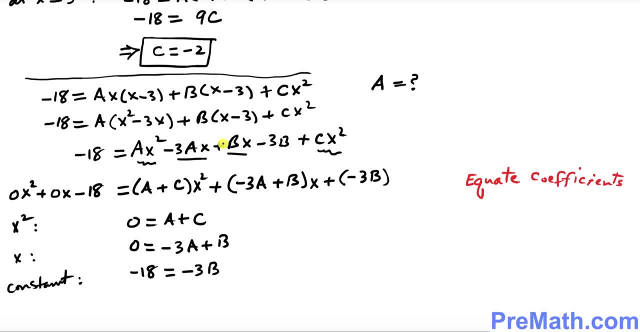 negative 3 B from these equations, as you can see over here, if you look at this equation, so a could be written as negative C and we know that C is negative 2. that means C is what negative 2. so I can write a times C, negative and. 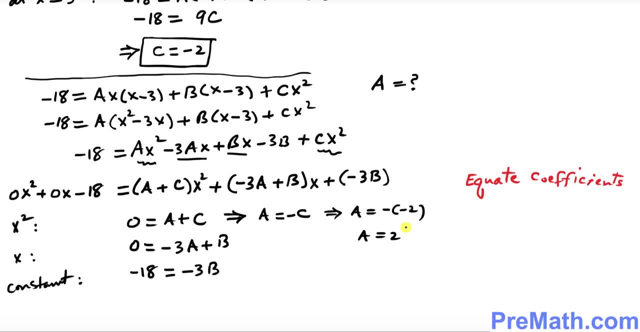 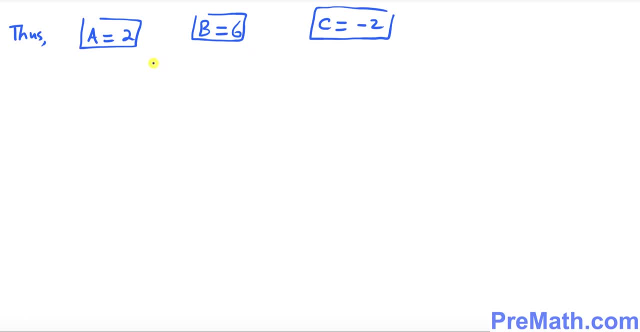 negative 2, so a turns out to be positive 2. thus our ABC values are right up here. we figure them out. so that's, our partial fraction is going to be simply a. whatever a is you replace is a by 2 and b replace it by 6 and c replace it by negative 2.